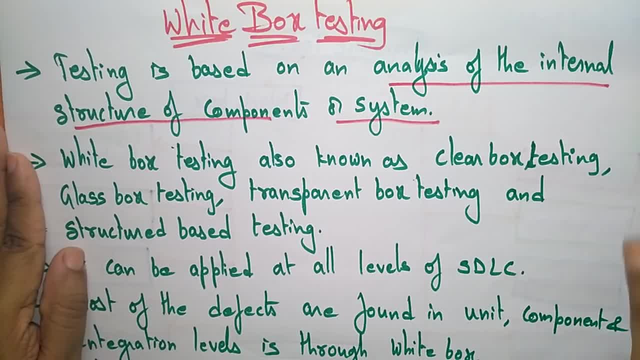 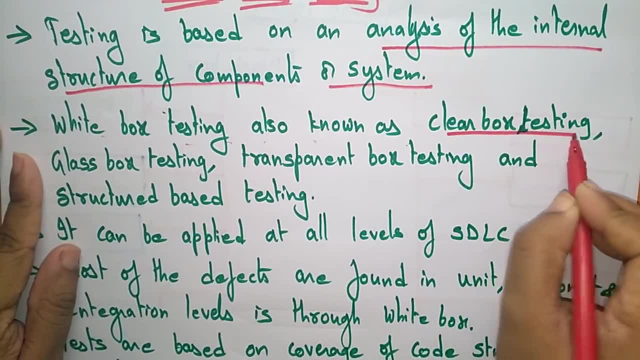 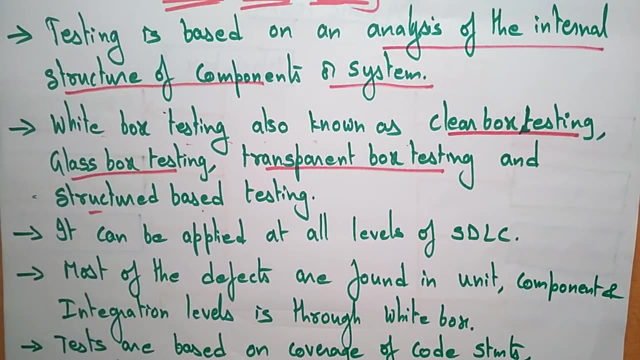 structure of: There only the structure and here the internal structure of components or a system. The white box testing is also known as clear box testing, glass box testing, transparent box testing And structured based testing. Why I am calling this white box testing like this? Because 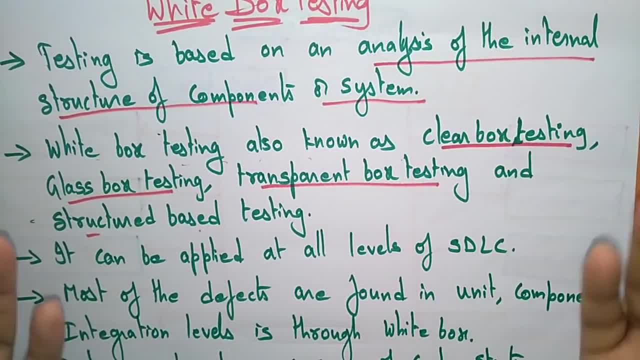 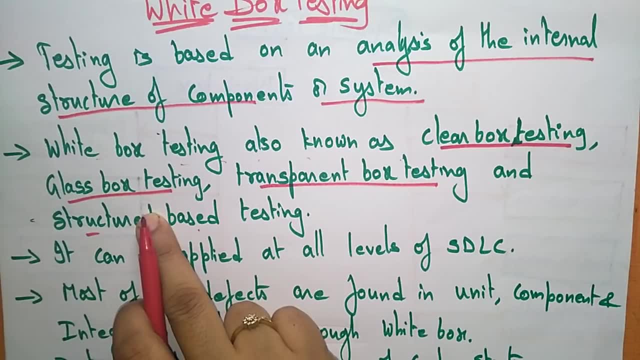 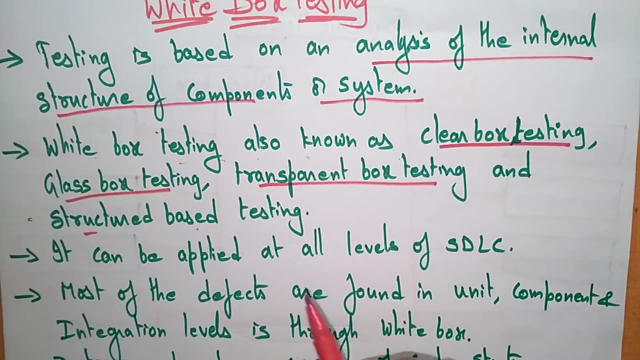 here it is saying: clear box means you are able to see clearly and glass box means in the glass. if you see everything. Okay, if anything is put on the glass you can able to see. and the transparent- transparent is also visible to everyone- means we are doing the testing on internal structure. 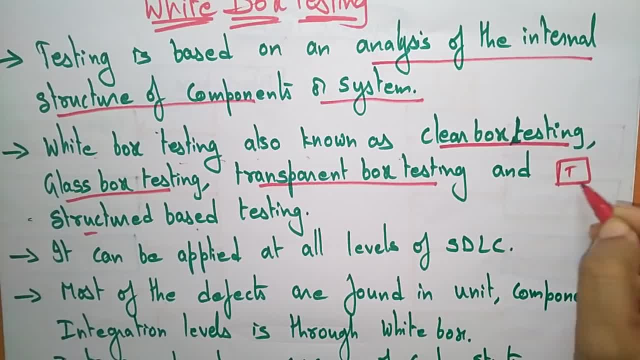 means it enter into the code. So whatever the code that is present, so it enter into that code and it is tested The integration, The integration internal structure of the system. so that's why we call it as a clear box, glass box, transparent box. 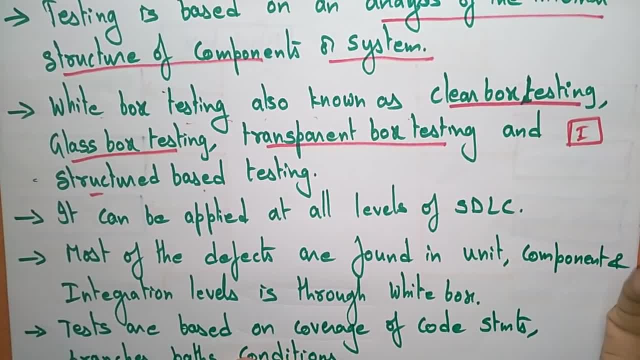 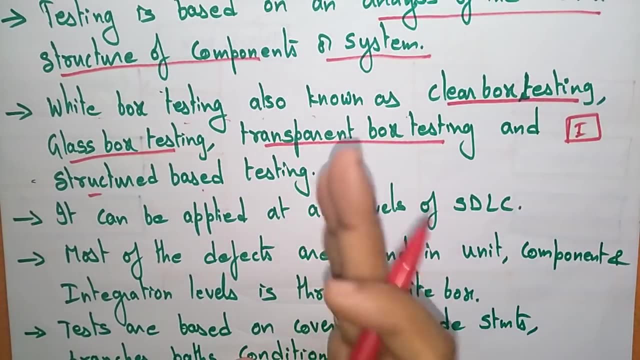 because, or whatever they're inside the means, whatever the steps that we have written and what are the programs that we have written in the for the product, so that will be visible to everyone. so that will be that is visible to the testers, not to everyone. i'm saying that, that is. 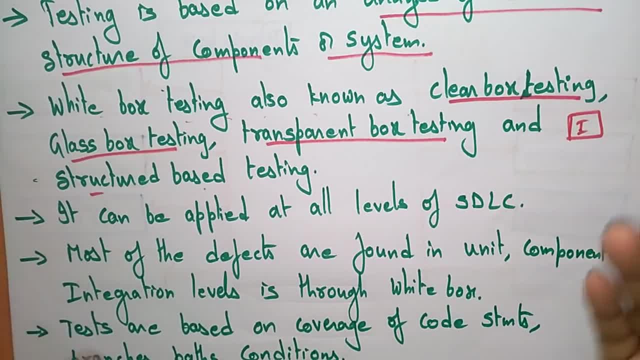 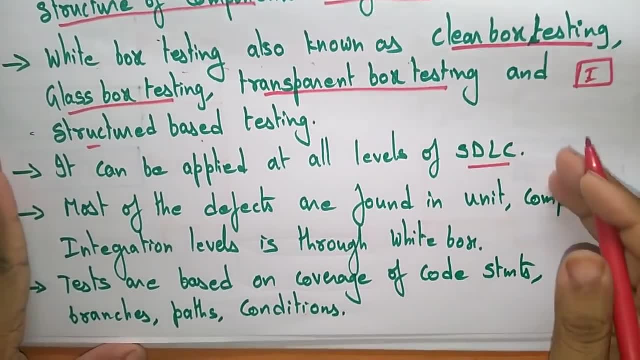 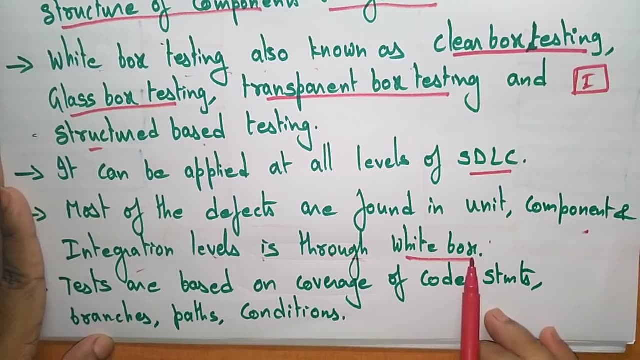 visible to testers. so that is a white box testing. it can be applied at all levels of software development life cycle. most of the defects are found in unit component and integration levels is through white box testing. so, uh, you will get. you will get an errors, okay, and most of the 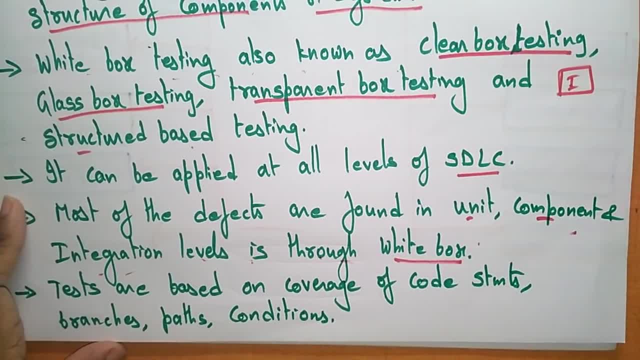 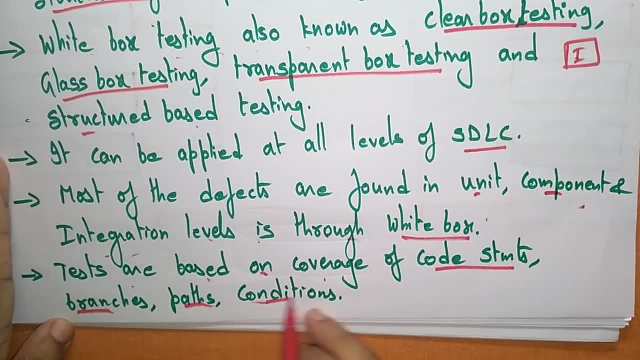 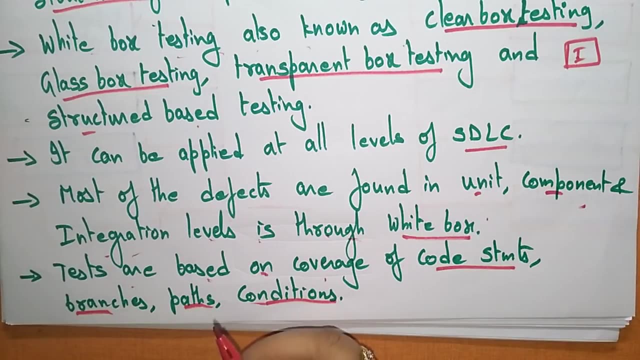 defects are found in unit, component and integration levels, test or based on coverage of code statements, branches, paths and conditions. okay, so if you're writing the code, the code code is completely based on the functions you're writing and the conditions that you're writing and the branches and the paths and different statements, that everything will be covered in. 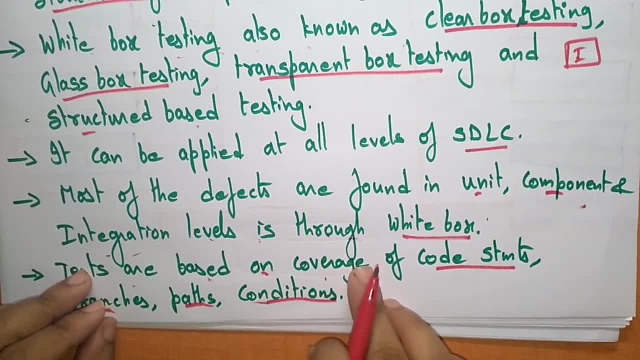 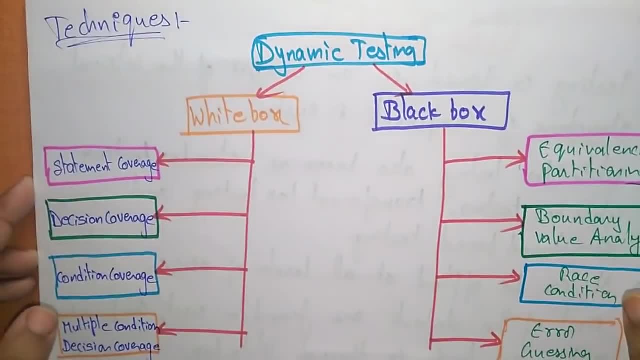 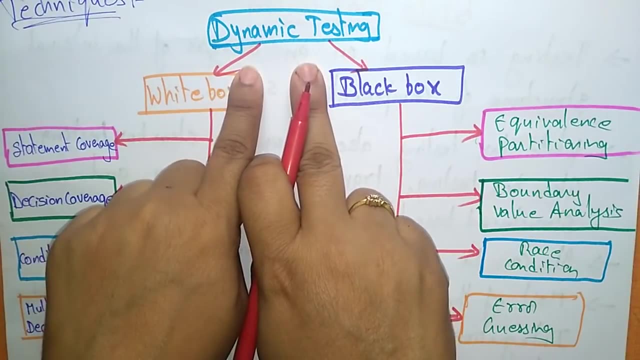 the program. so the test is completely on the, based on the coverage of code statements, branches, paths and conditions. now let us see the techniques that are present in the uh white box and the black box. so actually the white box and black box, both are the dynamic testing. we